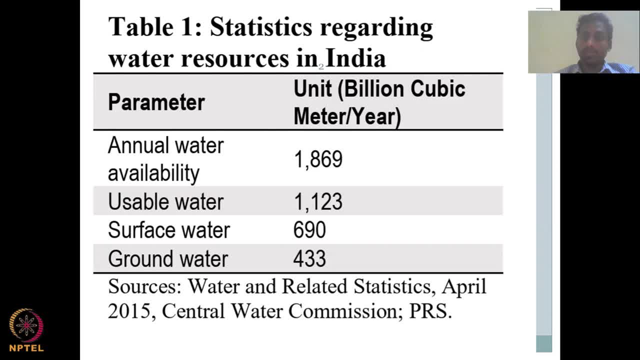 classes where we looked at the annual water availability as in billion cubic meters, We have around 1800-1900, close to billion cubic meters, of which usable is only 1100, or 1123 billion cubic meters, of which surface water is 690 and groundwater has a very good share of 433.. So what this clearly tells you is that of the 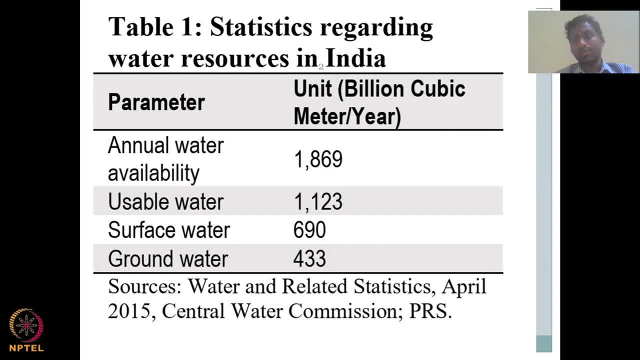 usable water. 433 billion cubic meter is supplied by groundwater. So, given all the rainfall, the storage, the big dams, still the groundwater usage is a very considerable amount in the annual groundwater use in India. It is also a very decentralized water wherein you don't need a channel, you don't. 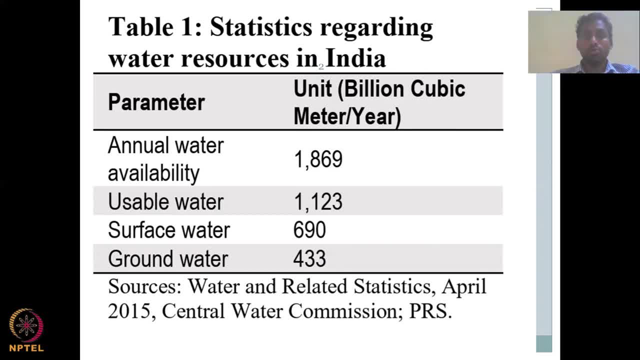 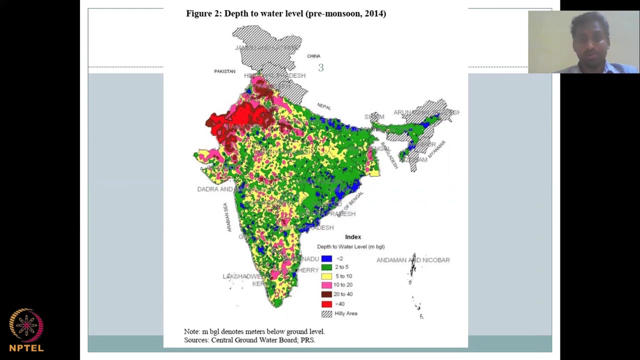 need a dam to store and then do it, but everyone who has access to wells and pumps can locally source the water. So, because of the ease, because of the access and technology, the stress on this water has also increased And it's been captured by different groundwater maps, especially the pre-monsoon, because that is. 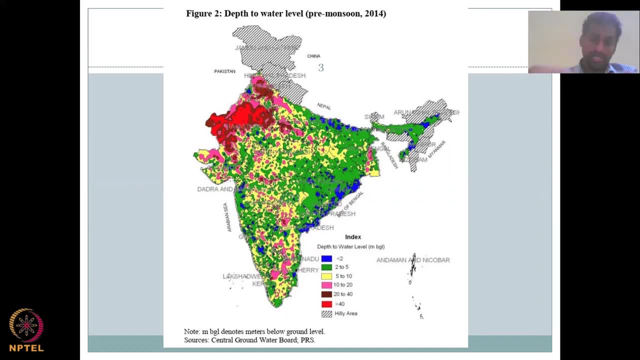 the peak summer. So after all the rainfall, after all the recharge happens, you extract water and it is reflected in the pre-monsoon season maps. So if you look at 2014 and you could see that it's been thoroughly disposed of by the four major land areas. So this is when 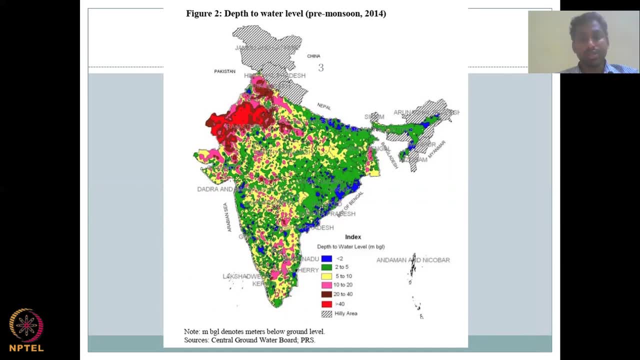 these JUG used water and these lands are all deficiencies for water use. So these areas are really especially out here in Central in India, where it goes five to ten meters, The yellow colour and pink colour 10 to 20 metres, but most importantly, Rajasthan. 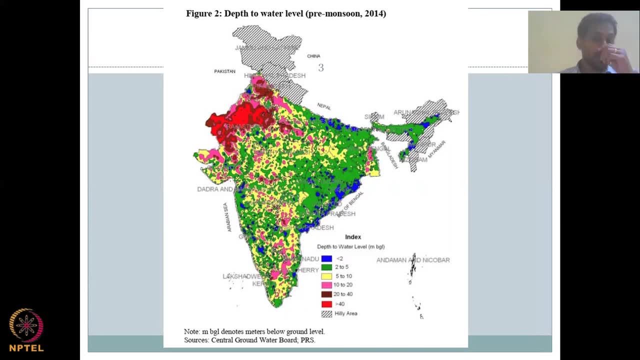 by agricultural activities. So agriculture has been a biggest consumer of groundwater and annually the water levels are decreasing in these regions. So it is not that okay, you're depleted and then it comes back again annually, but it's not. So there has to be some measures. 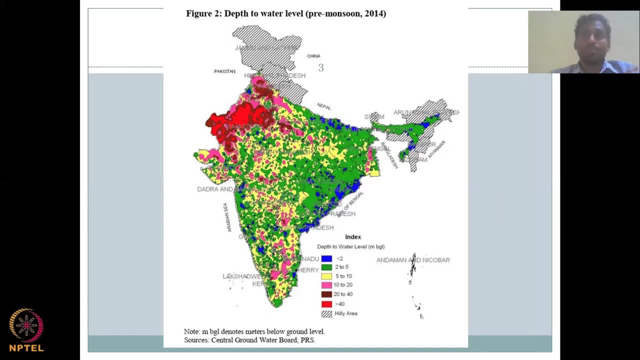 some stringent rules on groundwater use and abuse and more progressive thinking on groundwater. Also, a lot of people react later, very, very late. So by that time groundwater depletion has hit a level that it is almost irreversible. So it is more proactive measures are needed. 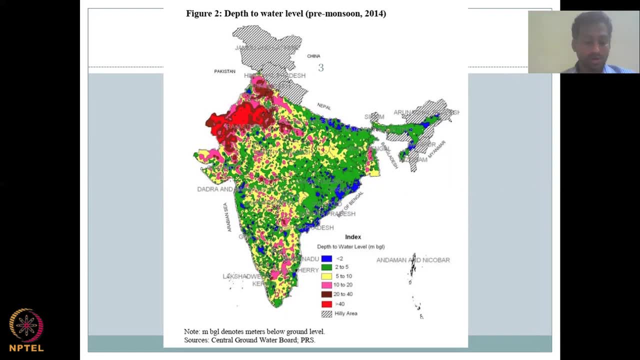 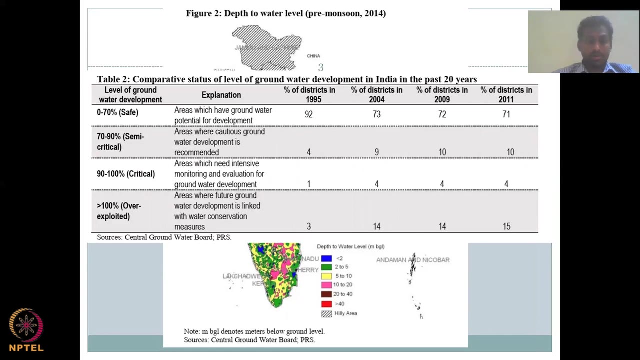 wherein, visualizing the groundwater use, visualizing the groundwater demand, we need to understand and develop methodologies that can recharge faster or limit the use of groundwater. Let's look at a table of comparisons And, as I mentioned earlier, Central Groundwater Board characterizes the blocks. 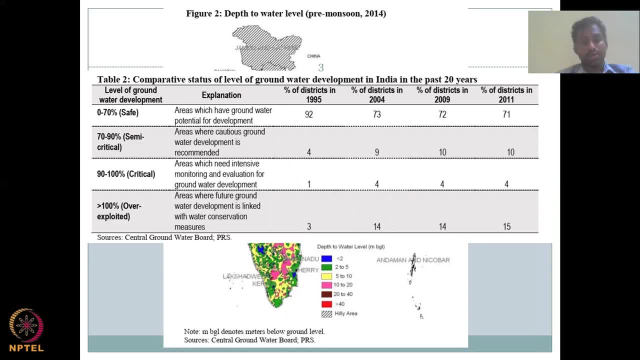 as safe, semi-critical, critical and over-exploited, based on the groundwater use. If they use zero to 70% of the annual recharge it is, you can still use some water and 30% could be given to ecosystem services. 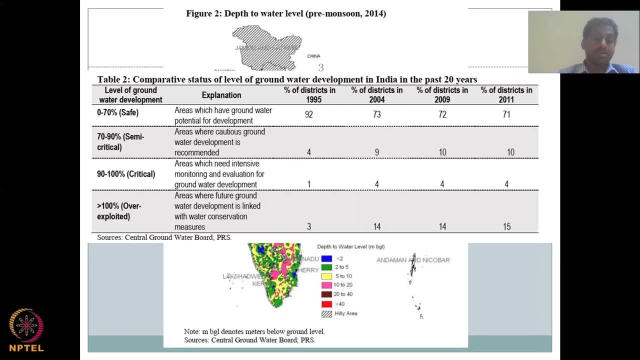 base flow, stream flow generation, et cetera. 70 to 90% is semi-critical and anywhere 90 to 100%, which means you are using the annual replenishable water in the groundwater. every year you're using it. 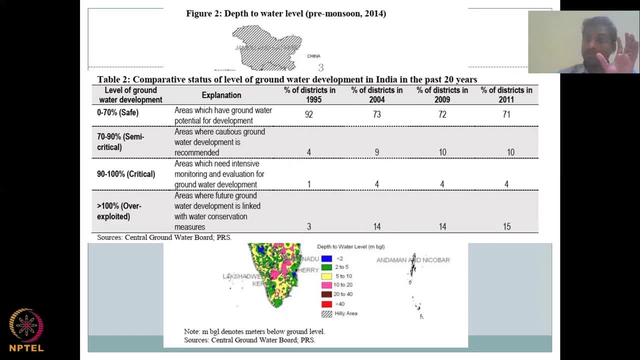 So think about your bank account analogy again. If you have 1000 rupees coming in or 10,000 rupees coming in per month as a salary and by the end of the day, end of the month, if you have zero balance, then that is critical. 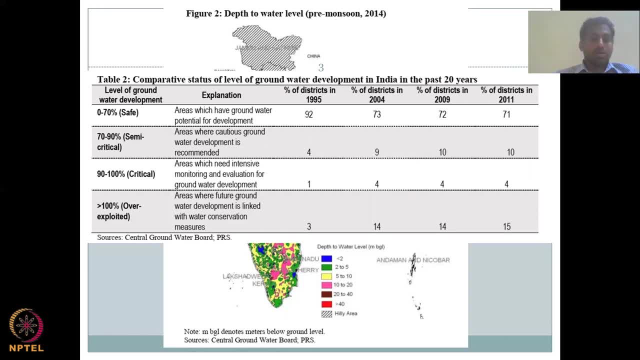 Because, if anything, it is critical, Because if anything happens, you don't have water, you don't have money. But 70 to 90% is semi-critical. zero to 70% is safe. Over 100%, which means you are using a past recharge water. 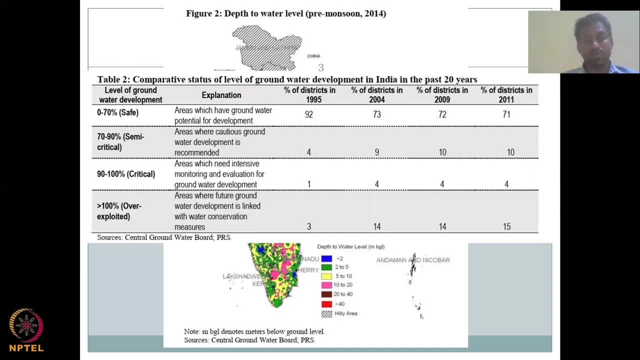 or someone else's water, So that means it is over-exploited. That is the concern. So over-exploited is the concern and critical is also a big concern, because critical stages can easily jump into the over-exploited. So think about a bank account. 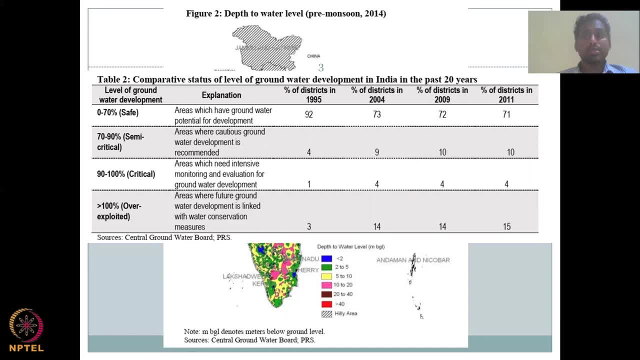 We have 10,000 coming in every month And at the last day of the month, if you say no, I need more, I've exhausted my 10,000 rupees. I use a credit card or a loan and I take more. 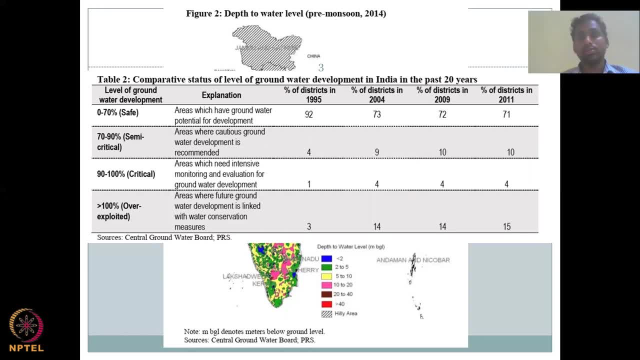 it adds up as a debt. Okay, so you are actually eating into your future water, or you're taking some savings and then using your water. So over-exploitation is bad. If you know the water levels, why would you go? and you know? 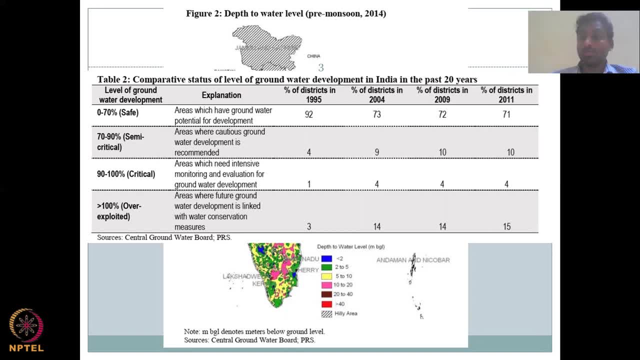 you're not going to be able to get water. You're not going to be able to get water. Use more water is the question. If you know you're going to get 10,000, you should have your demands and also your needs within the 10,000 so that you are safe. 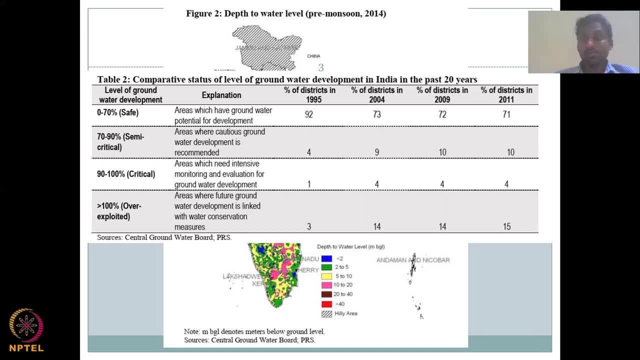 Otherwise it is over-exploited And that is not sustainable. How long can you do that? At one point you need to stop. Maybe you will say, okay, I want to spend that for some time. I can stop, But water is not that. 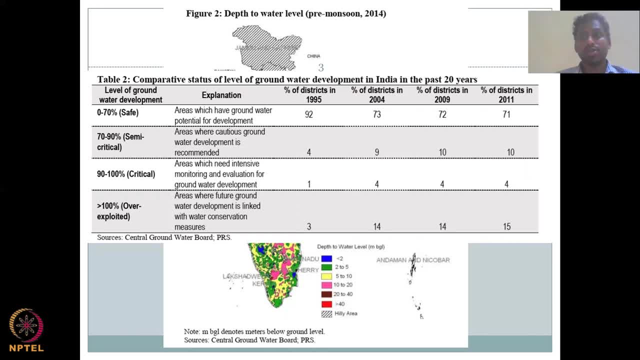 Every year you need water. Every year the trees need water. Every year the streams need base flow. So over-exploitation and critical stages are very, very important and groundwater board and government agencies working on arresting these groundwater falling levels by putting in more infrastructures or mapping them. 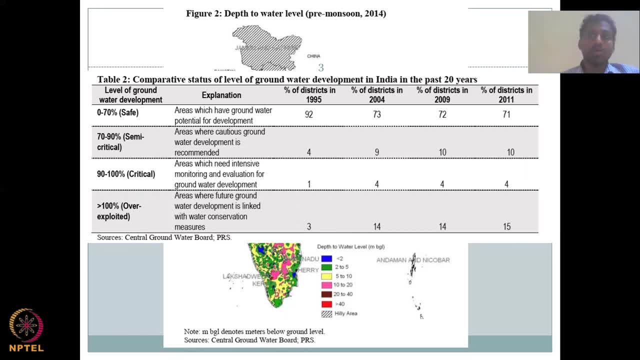 for the government records and sensitizing people on not doing these kinds of activities. The rules and regulations are not yet stringent, because it is very hard to understand Where the pumping is, who are pumping, et cetera, et cetera. 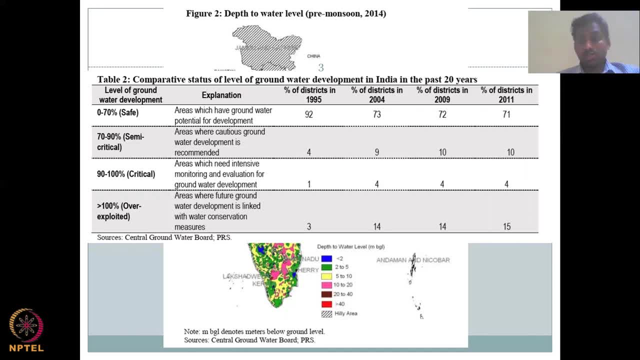 So zero to 70% areas have groundwater potential for development. So you still can extract more. And if you look across the years from 1995 to 2011,, the percentage of districts in the past 20 years shows clearly that the safe level blocks and districts. 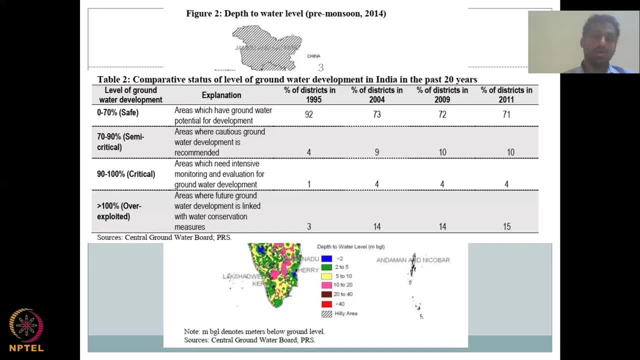 have come down, So 92 to 71, okay. So look at 1995, it was 92 districts were safe. 2011,, 71, which means your safe districts are coming down, Whereas your over-exploited and critical are increasing. 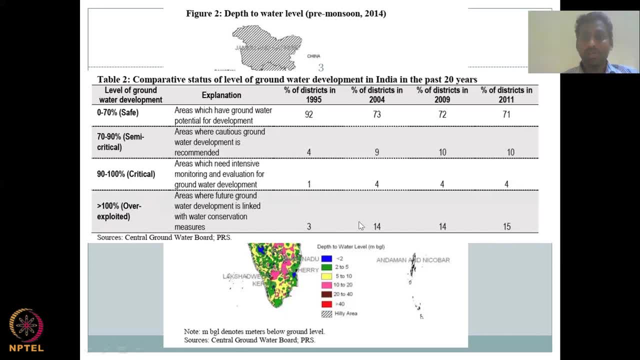 Especially your over-exploited, which was three. it jumped to 14,, 14 and 15.. So within 10 years you have 14 districts over-exploited. Same in the critical stage also 1,, 4,, 4,, 4.. 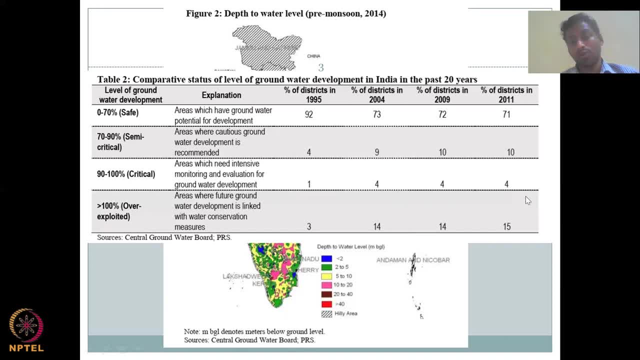 So what do you see clearly is the safe and semi-critical have been converted as critical and over-exploited. So this is why I'm trying to say that critical blocks, critical districts, have to be managed with utmost care because they can any day become over-exploited. 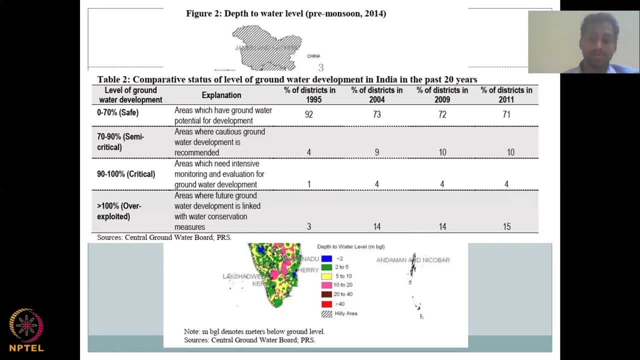 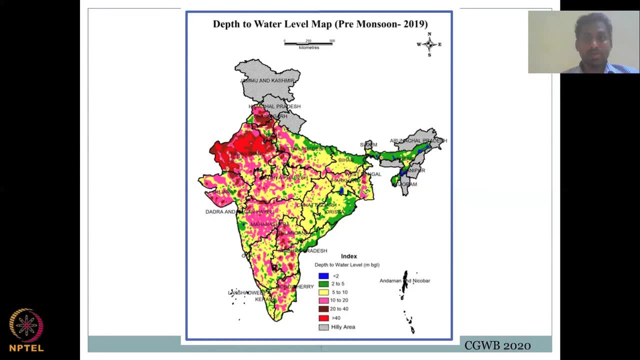 Let's look at how it looks now compared to 2011,, 2010, and 2015.. So here is the state of the state of the state, Let's see, Let's see, 11 images. so in 2011 images you saw a lot of green color here. let's go back and show you quickly. so. 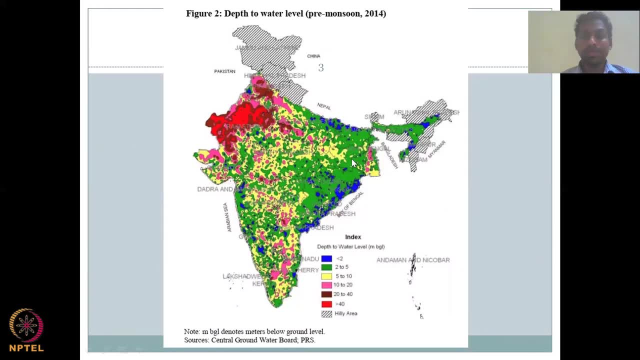 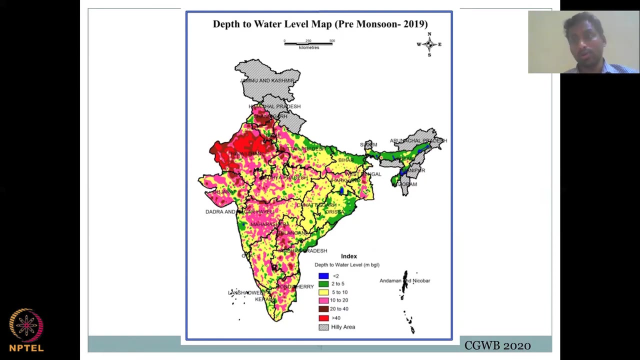 you saw a lot of green color, which is two to five meters depth. uh, to the water level, which is still safe, and five to ten. ten to twenty are really bad. blues are okay, but when you come to print 2019, which is the latest 2020 report image, you see clearly that, okay, the borders of the green. 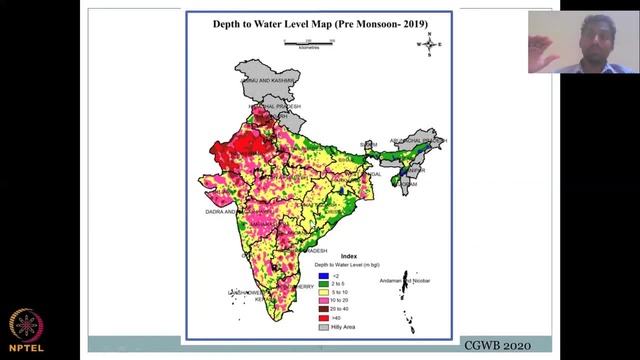 are still, but the central india is actually coming levels. it is the same legend, so the coloring is the same. so two to five, which were here, all the green colors, all the green colors along this region, central india, are now in the 10 to 20, not even 5 to 10.. so you have jumped. 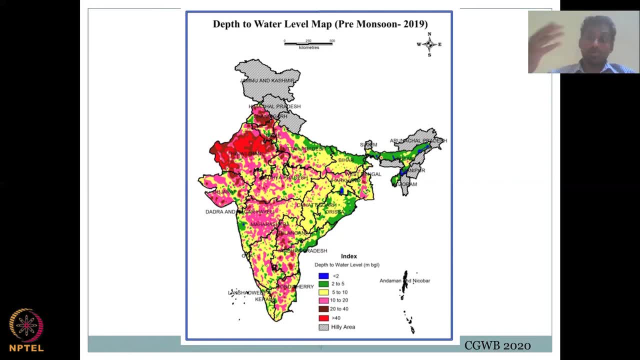 15 meters from your 2011 level. so within eight years, or even nine to ten years, your groundwater has fallen by 15 meters, and that is not sustainable. multiplied by the area, you would understand how much volume that is, which is very, very big compared to the water volume available. 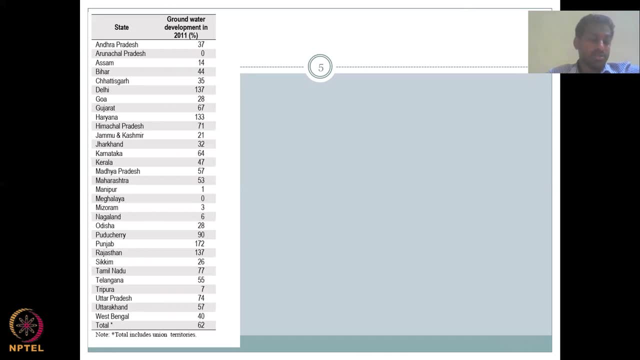 let's see which are the states. you saw the districts. now let's see the states, which are states that are using very high amounts of groundwater as person development, and i said anything above 100 is bad, but we'll still put a ballpark around 90, which is so 90 and above is not acceptable because it's. 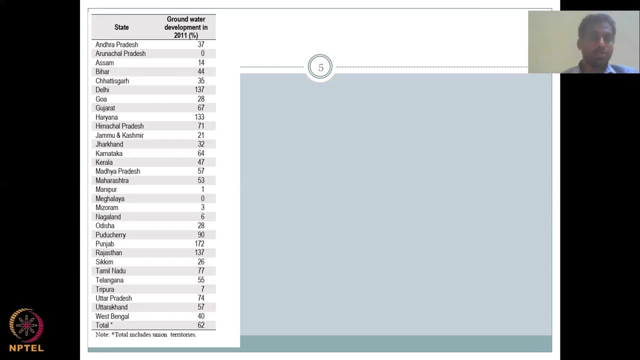 very, very um harmful to the groundwater aquifer. so you can come down to delhi. delhi's water is the fasto眼 is a water fiction action TWO U ZI SOFTcart which will lose a lot of water around 90% on this upper on now and in post you regret thatента is wow탕. water in delhi is is on top of the city and then midway sense on here you. 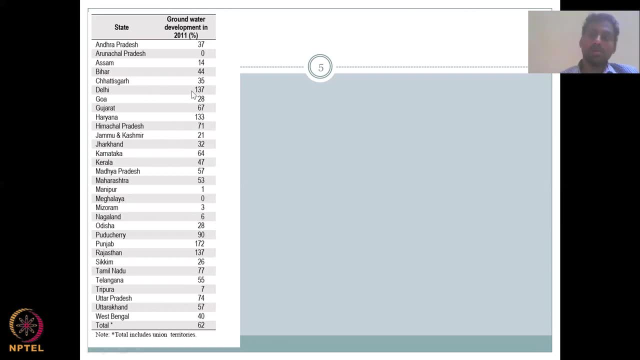 cte ym is groundwater levels are above the recharge. So the use is above the recharge and the government is working on a lot of methods to bring back the water by recharge and other mechanisms. but the population is very high So there's a lot of groundwater use. 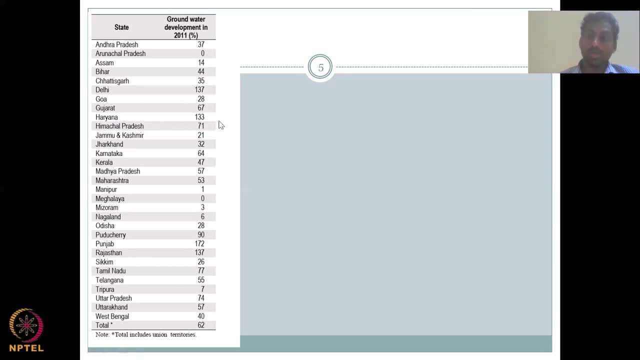 Coming to Haryana, which is an agricultural state, you could see the groundwater use is above your groundwater recharge, because 100 is equal, Groundwater recharge is equal to groundwater use, but here it's 133, so 33% above. And when you come down another 90 is Puducherry. 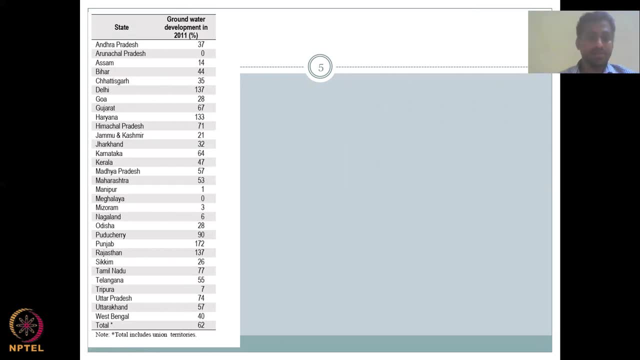 a very small state. There's a lot of agriculture activities there and also urbanization. Punjab is purely driven by agriculture and you could see a lot of agriculture activities supported by groundwater, So groundwater has to be managed as much as possible. So there's a lot of work to be done. 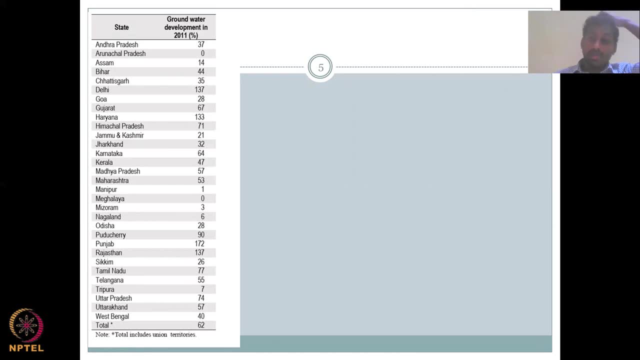 to make sure that the groundwater is as much as in Rajasthan and other states. So all these states in 2011 have performed kind of on the critical or semi-critical levels and the handful which are on the over-exploited, but in recent years the levels are not promising. 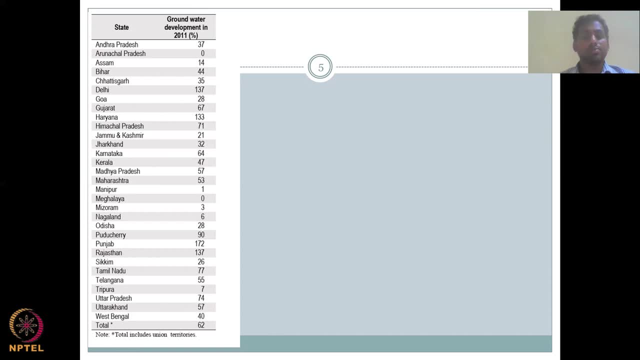 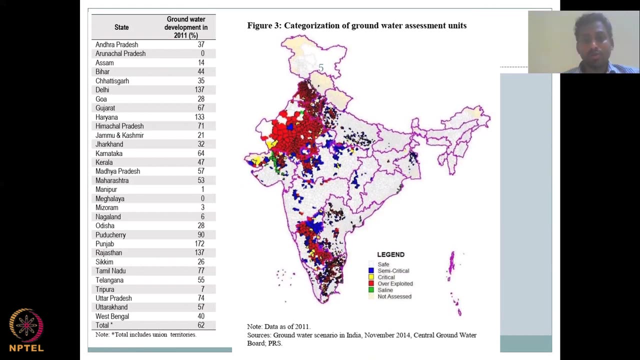 because everyone is now having easy access to groundwater, And so these are the characterizations of the blocks of semi-critical, say, critical and over-exploited or over-exploited are in the red colors And you could see in 2011,, most of it. 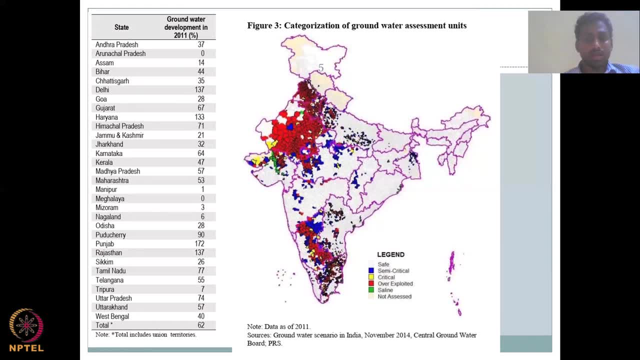 is in Haryana, Punjab, Rajasthan. There are some blocks. so compared to the district, there are some blocks. So within the district, the image might not be that helpful because part of the district is urban, part of the district might be a desert. 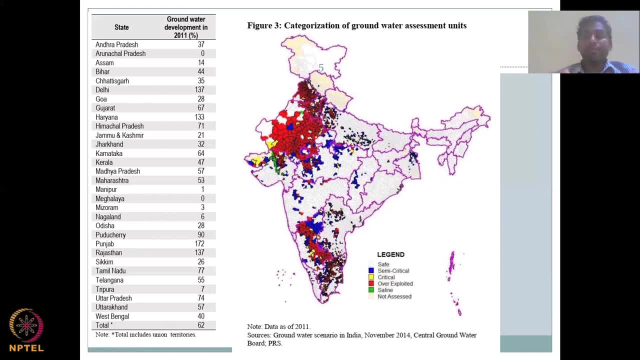 part of the district might be a forest. So overall, averaging a district might not be that helpful, but a block image actually shows you where the water is being used more than the recharge, And now you could see more. southern states have blocks that have high demand in groundwater. 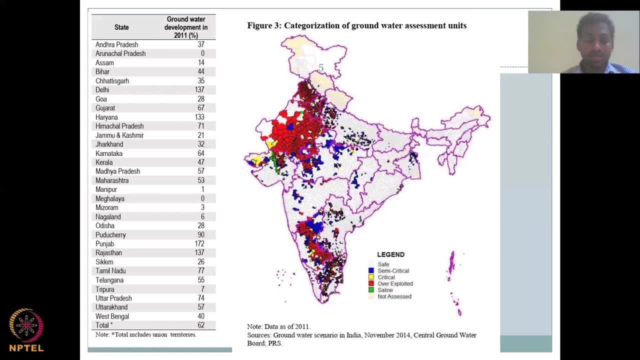 Bangalore, Chennai, all the big cities are there- Hyderabad, et cetera, et cetera. The reasons: okay, leave the urban reasons. Let's look at the big, big states and big, bigger blocks. What is the reason? 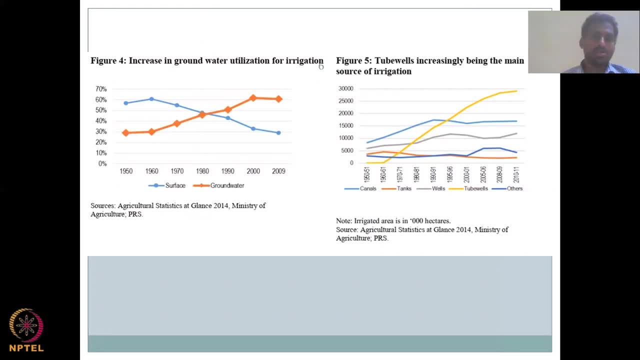 It is agriculture, So increase in groundwater utilization for irrigation has tremendously increased over the years. If you look at the agricultural statistics 2014,, you could see that the groundwater component in agriculture has increased from 30% to 60%, whereas the surface water has come down from 60% to 30%. 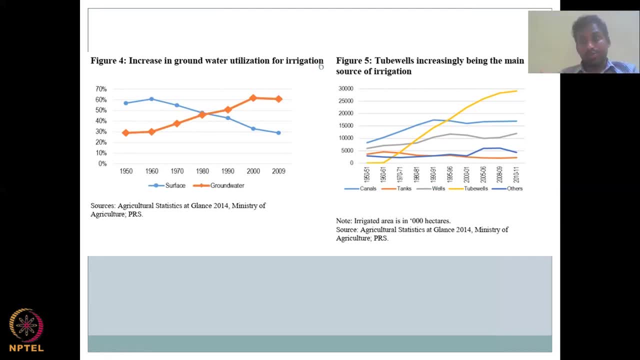 So almost it is exchanging their responsibilities. Okay, groundwater has been promoted as the key resource in those regions where surface water irrigation was happening And that again, as I said, surface water is a more centralized approach, where you have a dam and the dam releases water to farmlands, only to the farmlands where it has. 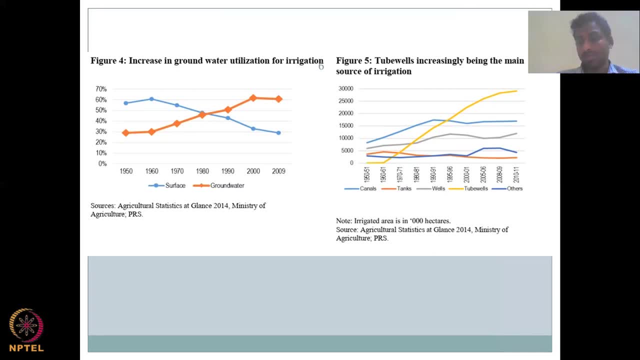 access to channels, whereas groundwater is. you just have to put in a pump and then suck all the water out, So coming back. so groundwater has overtaken surface water in some regions. but, more importantly, the pattern is exchanging between themselves. So the role, the responsibilities, 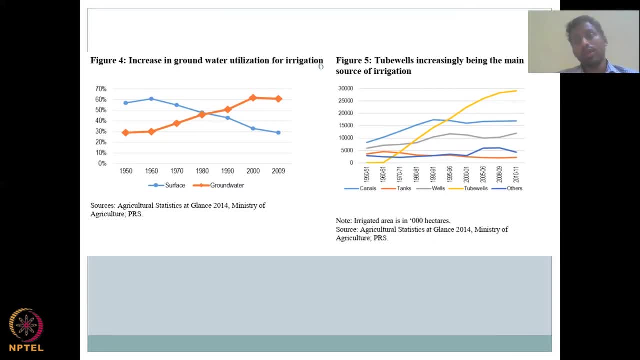 have been taken up by groundwater and more and more areas are coming under groundwater irrigation. The other figure shows another story: Tumors have increasing becare. So that actually is an indicator of the groundwater being the source of irrigation. So if you look at the source of irrigation, 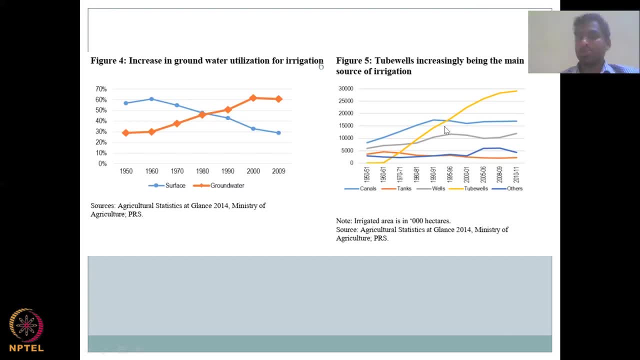 canals, which are surface water related, have almost stagnated from 1950s to 2010-11.. Tanks, also as a surface water storage unit, has also stopped or even come down in recent years, whereas wells have increased and, most importantly, your tube wells have just skyrocketed. 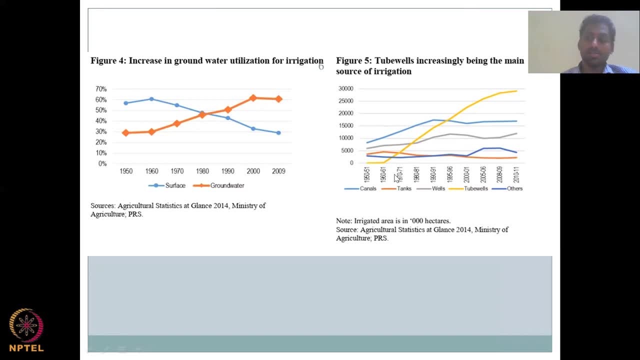 It was zero In the 1950s, 1960s. technology was expensive. There was not much development on groundwater pumps. but then, slowly, science and technologies have a prolonged effort in bringing up the groundwater pumps- electric pumps, diesel pumps, those kinds of things- And you could see a skyrocketing increase in the number of tubes. even the easy access and installation of tube wells has 484, Betty пропel: 52 years have. the app was set up by now three years ago, 1922 canals, or set up 50 new results are still capacity to 50 million and they're being upgraded every day, Even though this step is mostly Warm up. for the und offline at 50% render efficiency for wastewaterMPT. it may not allow many next to a $100 per dollar per meter to national map revenue. two of them have been posting anereal stocks for water collection softwares as variables, estratégica and waste disposal of from Georgia farmlands. 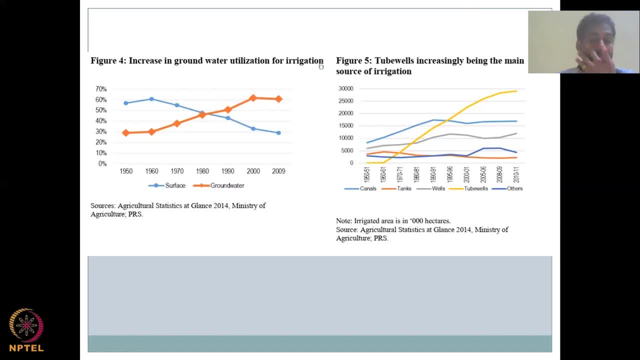 even the easy access and easy installation of tube wells has a big impact on the groundwater use for irrigation. So all this is not sustainable because initially one village would have two, three wells. I could imagine in my younger age when I was traveling in the villages. 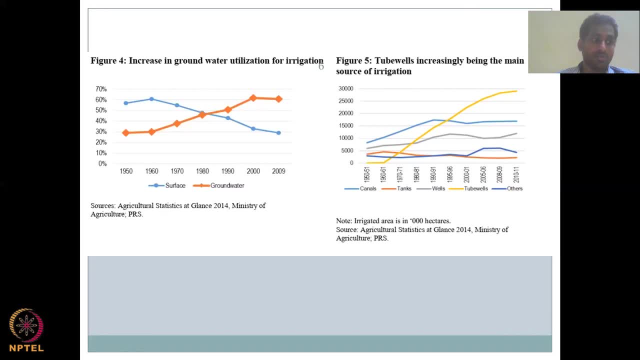 you could see only certain number of wells for irrigation. but now every small plot has its own. well, okay, Because there are some funds, there are some subsidies given and water is just being exhausted. But there is less and less groundwater recharge activities happening. okay, 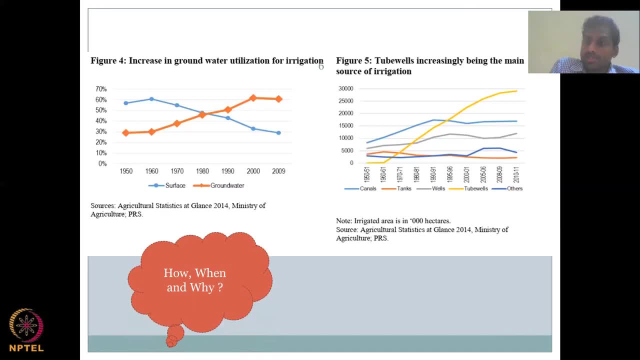 So how, when and why? What is the reason for this tremendous increase? Because there's a lot of stress on farmers to produce more food. The population is ever increasing and the weight falls on the farmer's shoulders because they have to feed the crops. 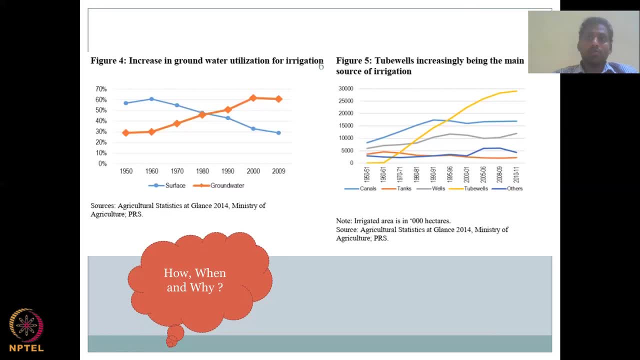 And also if they cannot allow the land to go fallow because of the technologies and hybrid products, so they would just put in more and more crops, fertilizers, All these things have actually converted the land from a single crop rotation land into two or even three crop rotation lands. 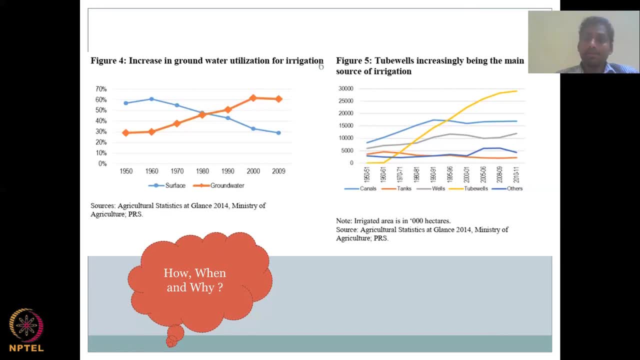 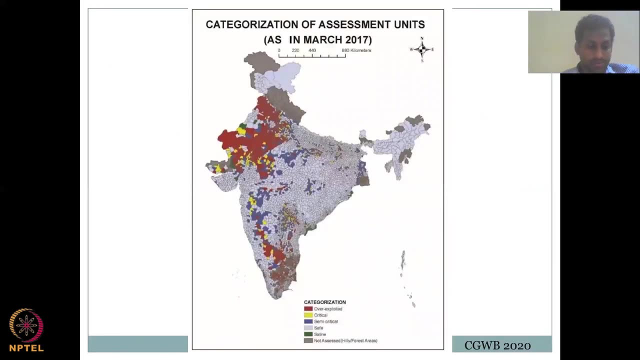 And with this rotation, there's more need of water and groundwater is being used, Because always you don't have rainfall for your karif season. Because of this, compared to year 2011,, you'll see more and more red blocks, overexploited. 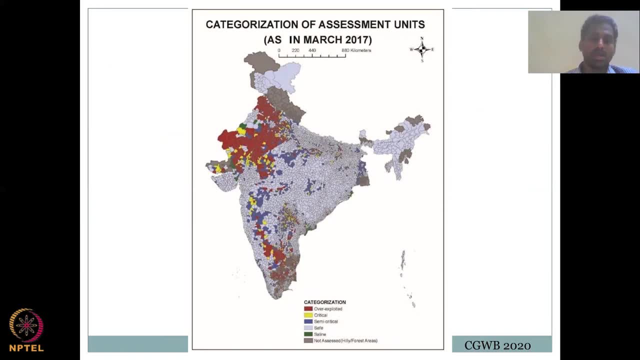 Especially in the north northern regions. But I would say that the ground reality might be much, much different because, if you go back to the issues and concerns I mentioned for groundwater monitoring, some of the wells are not representative Or some of the wells are not pumping wells. 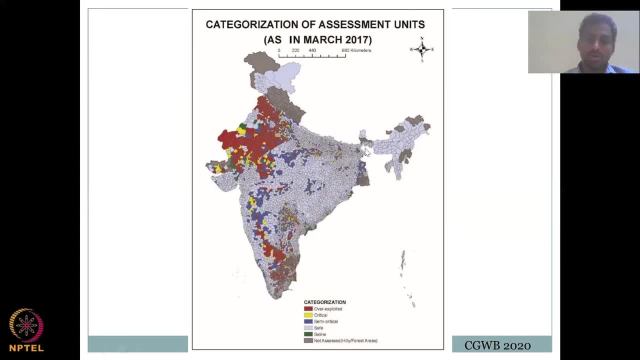 It is monitoring wells. And if you come to your central part of India, this is where we tie up all the learnings from these two lectures on groundwater hydrology. What did we find In the central part of India? it's sort of hard rock aquifers. 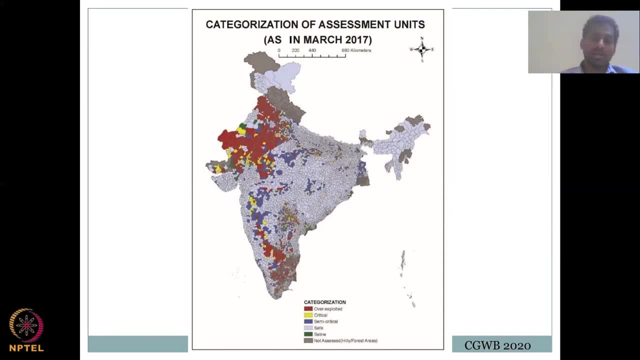 And hard rock aquifers are not well connected because it has fractures and some of the wells would not be applying together. it won't tell the same story. So if you have one well which is pumped for farming and right next to it a well which is not being pumped, 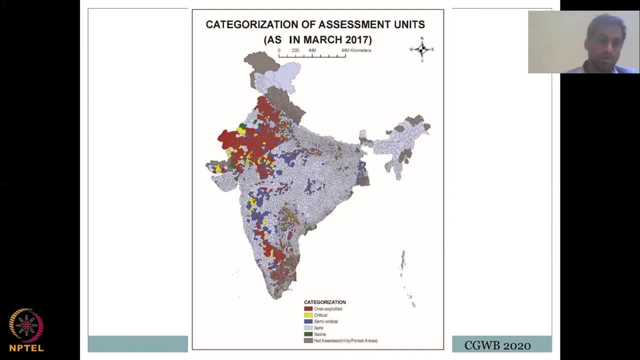 the water level will be always the same. So when you do a block estimation you might be misguided. So there is a more, more need for augmenting groundwater data with other data to understand the reality of groundwater use. So if you look at the papers, 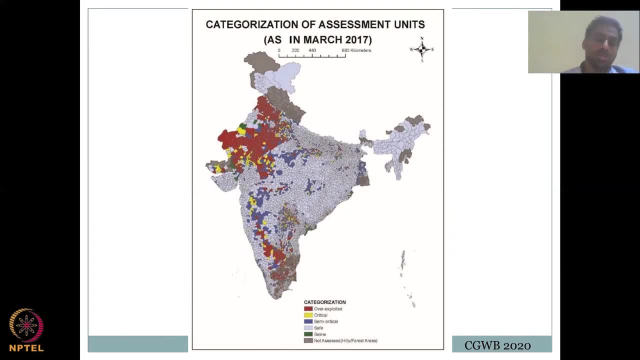 and other things that will be shown in the case study approach. in the following lectures you'll see report, sensing images and also land use, land cover, use data- all these combining to give a groundwater estimate, not just a groundwater level, okay. 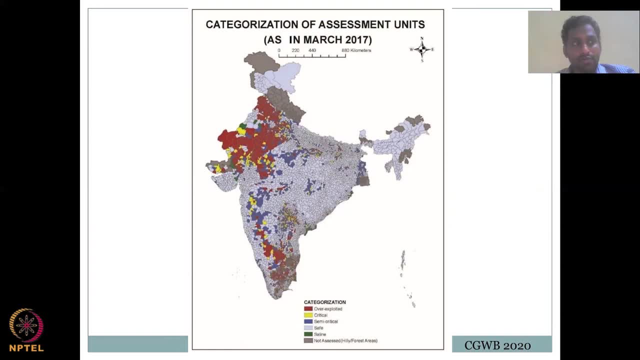 Because, at the end of the day, if you have a land full of crops in a non-rainfall season, how did the crop grow? You should have given groundwater right. So that is where you link the groundwater level with rainfall. 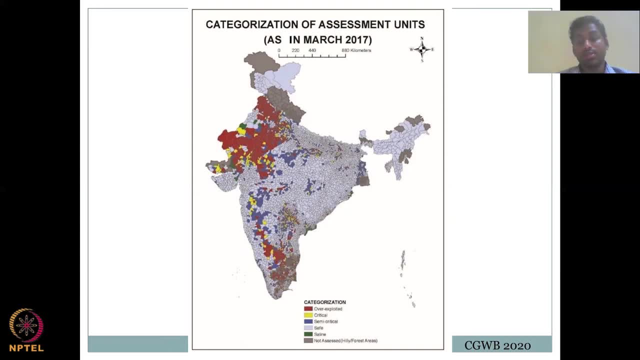 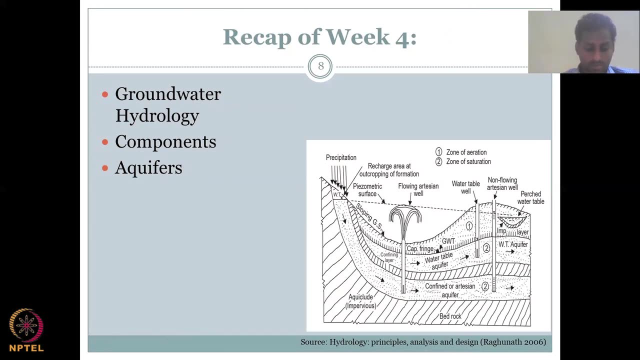 with your land use and cover change to understand what is the reality on the groundwater. So with this let's do a recap of week four. We did do a very focused discussion and learning on groundwater hydrology, where we focused on the overall hydrology. 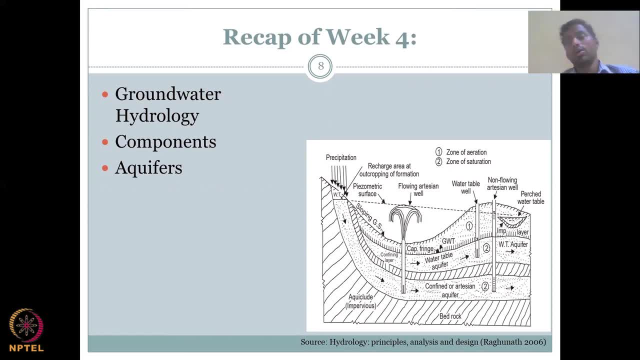 only the components which are necessary for groundwater. We looked at the most important components of precipitation, infiltration, and then how water moves down in the soil profile to different compartments in the aquifers, et cetera. We also looked at the very important material. 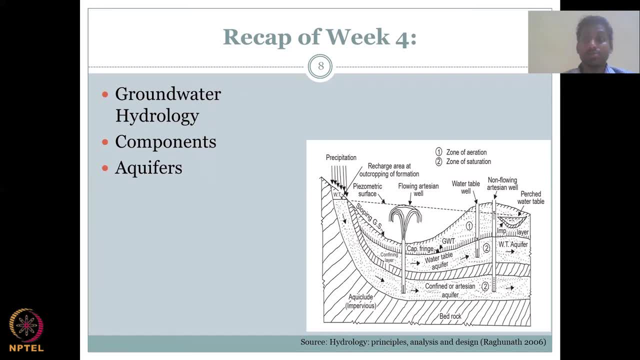 and material properties for groundwater hydrology, which is basically your sediment and soil materials, along with the porosity, the pore, space where water can enter and store. So these components. we looked at many illustrations and we understood that if there is a confining unit, 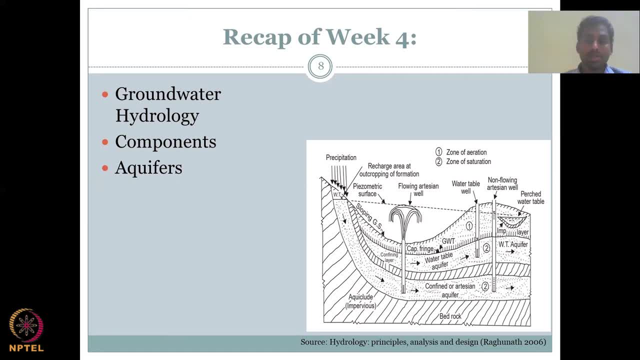 or a impervious layer in between the aquifers. then the aquifer is divided as an unconfined and confined aquifer. The unconfined aquifers have the top surface, the open to infiltration, precipitation coming in, whereas the unconfined are having 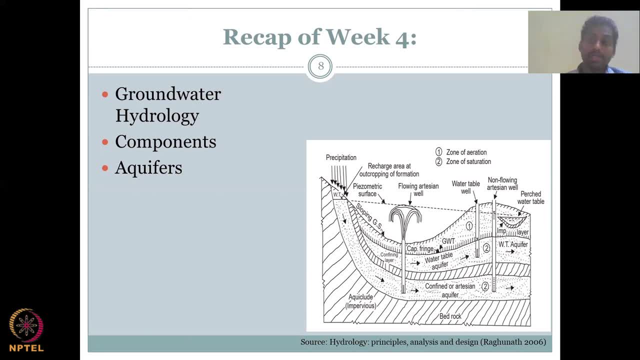 a confining unit both on the top and the bottom, So any system can have only one unconfined aquifer. but the confined aquifers can be multiple And, depending on the placement of your wells and the depth of the wells, the wells get different names right. 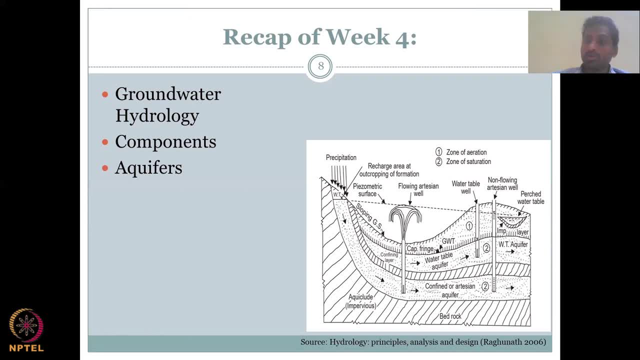 So if you put a well in your shallow aquifer, you will mostly be a dug well or you will have a well with a 30 meter depth. so it is annually recharged. okay, Shallow aquifers are annually recharged. 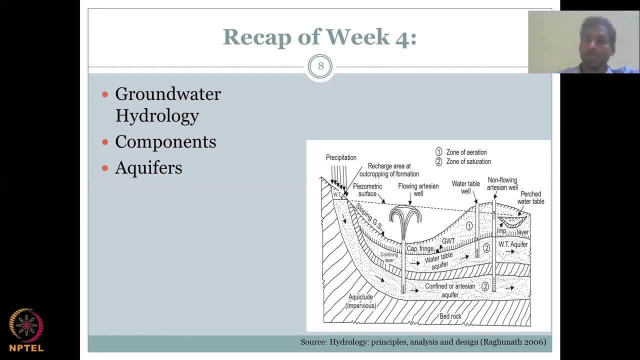 or even within a couple of years. we looked at residence times, we looked at recharge times, et cetera, when we discussed about aquifers. When we have deeper aquifers, this is the bigger concern. your deeper aquifers are going deep into the system. 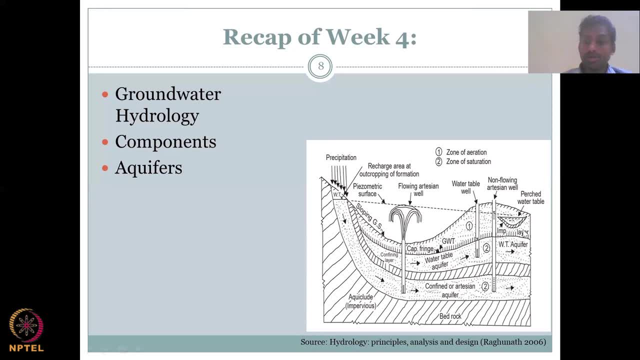 like here and it is clean. so it doesn't take water from the shallow aquifers. it takes only from the deep aquifers and you are using water which has been stored there or taken time around a hundred years or even a millennia, a thousand years. 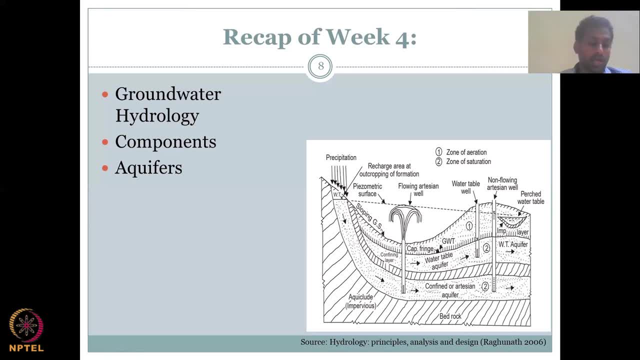 for the water to come there. So if you deplete it you will have to wait another a hundred years for the full aquifer recharge to happen, which is not possible in one's lifetime. So with utmost care and concern aquifers should be used, especially the deep aquifers. 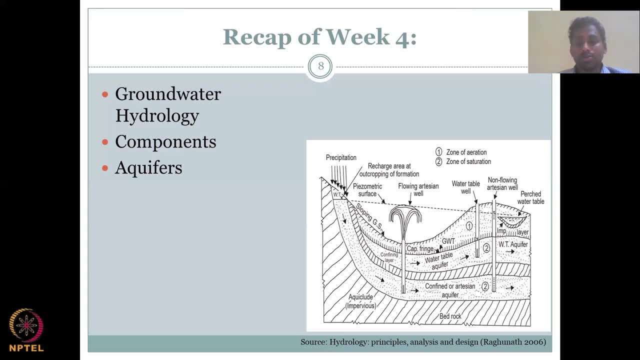 If the shallow aquifers are depleted, then you know you have to wait another hundred years and you have to wait another hundred years and you have to wait another hundred years and you have to wait another hundred years. then multiple opportunities are there. 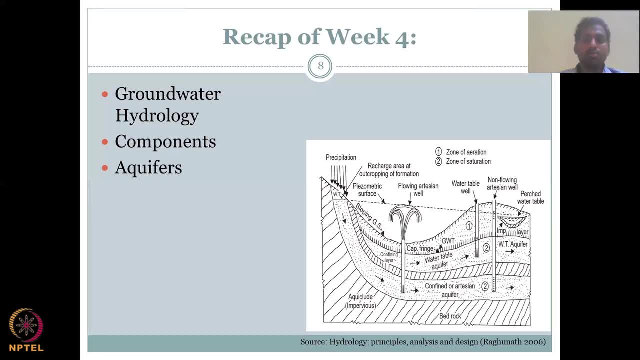 to enhance the groundwater recharge, which we'll be looking at in the coming weeks. But, more importantly, you'll be looking at how water structures, both natural and artificial, can aid in groundwater and surface water hydrology for rural development. We also looked at zone of aeration. 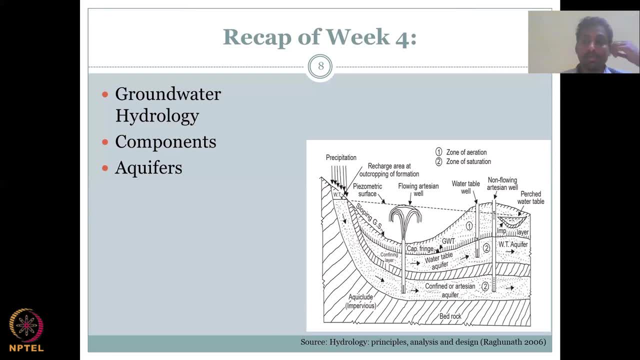 versus zone of saturation, where there's a zone where it has, where the soil has pore, spaces still without water, or void spaces. without water are called zone of aeration because air is still present, Whereas zone of saturation is the zone where the void spaces are filled up with water. 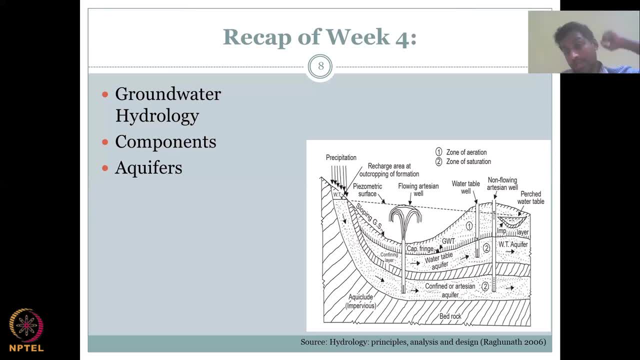 So all these things we looked at, and we looked at the sloping nature of the land which helps in groundwater movement laterally, And we also discussed the stage where groundwater recharge happens and it goes until your last impervious layer, which is your aquilude, aquitard, or your bedrock. 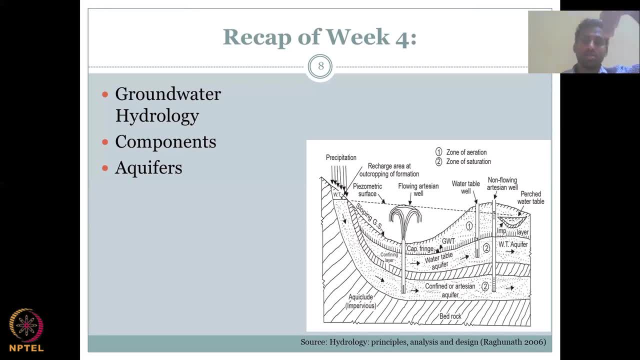 And after that water. even though gravity is acting on it, water does not move down, but laterally, And once it goes laterally there is a natural discharge. So discharge can happen in multiple ways. You can put a pump and take the water out. 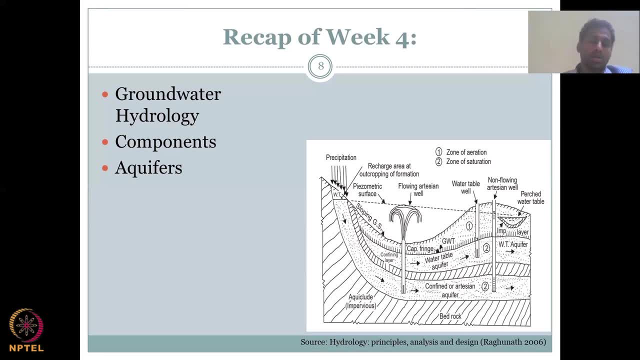 That is your artificial discharge. but natural discharge is when groundwater goes and at one point comes out of your lithology or the earth's crust into the streams, rivers or springs. We also looked at perched water table, which is very less in number, and artesian wells, which are less in number. 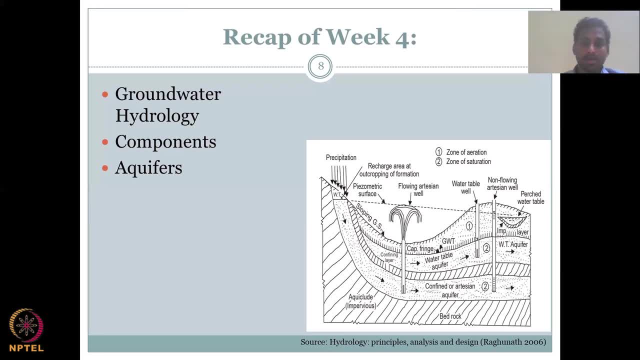 and what are the reasons through which it happens. We looked at central groundwater data, how it's collected, and other measurement devices, And the driving force here is: the data is present, but to have more understanding and more management plans, there is a need for augmenting these observation data.